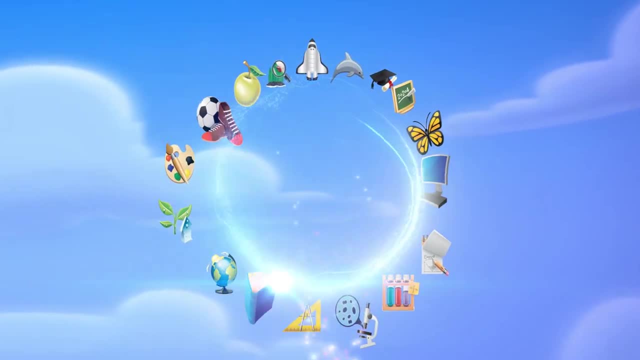 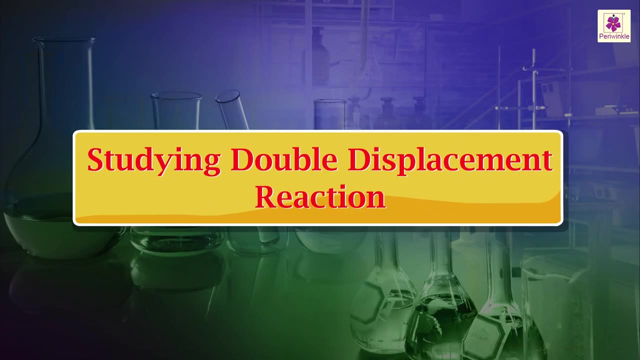 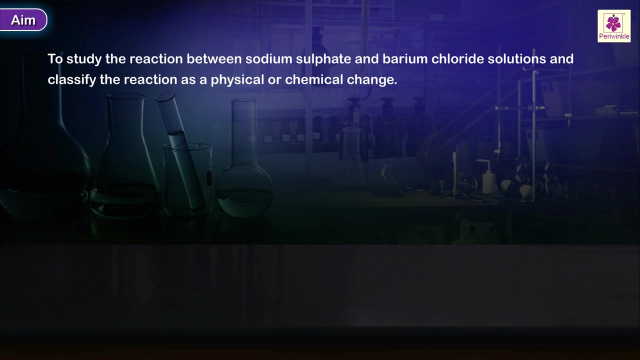 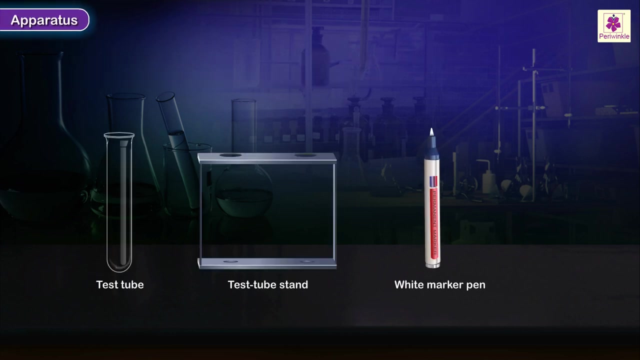 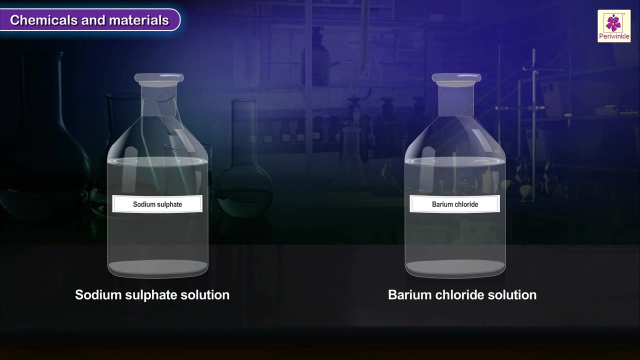 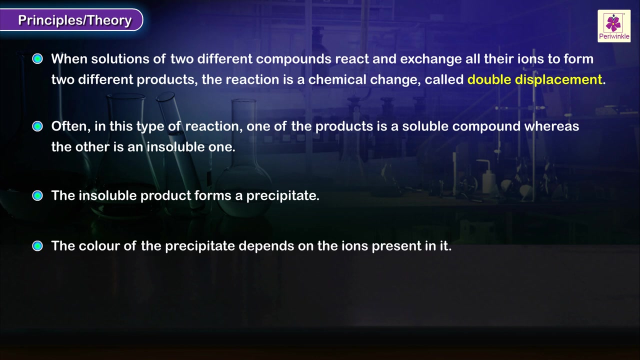 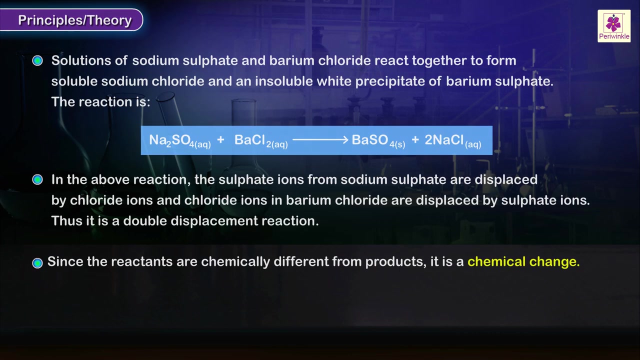 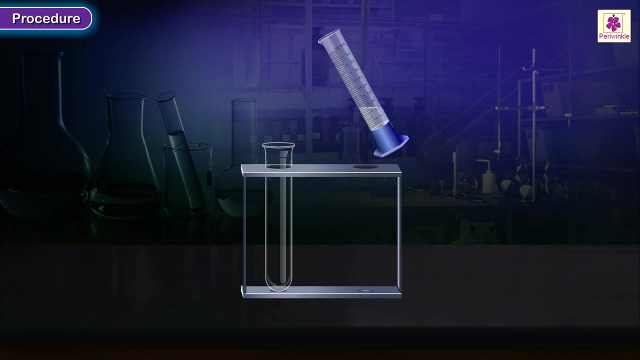 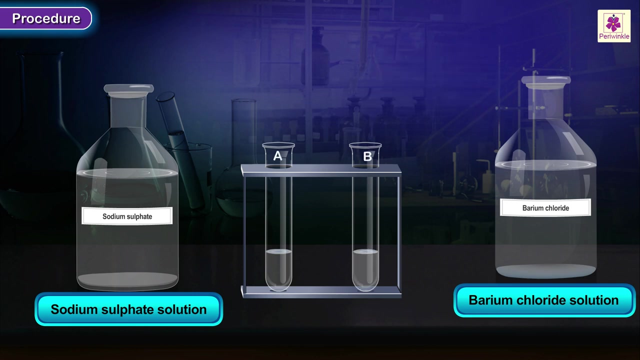 Studying Double Displacement Reaction. Aim To study the reaction between sodium sulfate and barium chloride solutions and classify the reaction as a physical or chemical change. Apparatus, Chemicals and Materials. Principles, Theory. Procedure: Take about 5 ml of sodium. Place the solutions of sodium sulfate and barium chloride in two separate test tubes and label them respectively. 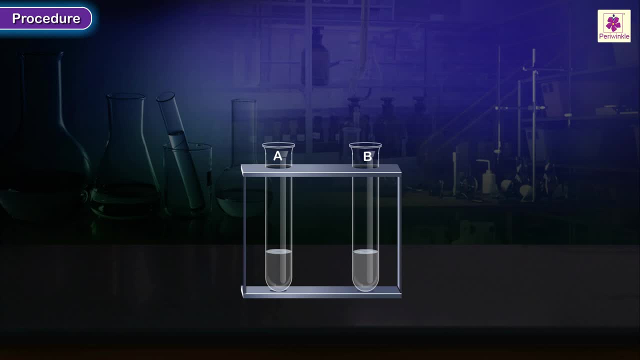 Place the test tubes in the test tube stand and observe the color of the solutions. Observations and Inference Solutions of sodium sulfate and barium chloride solutions are the following: To study the reaction between sodium sulfate and barium chloride solutions and classify the reaction as a physical or chemical change. 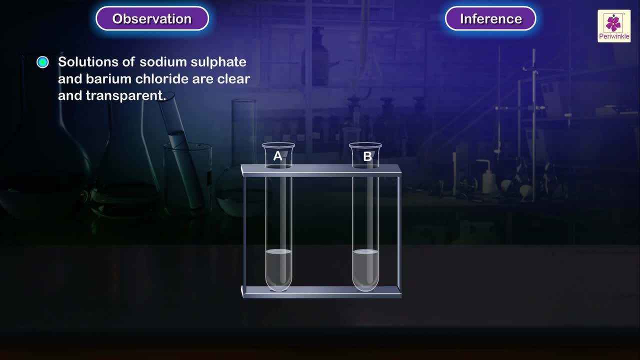 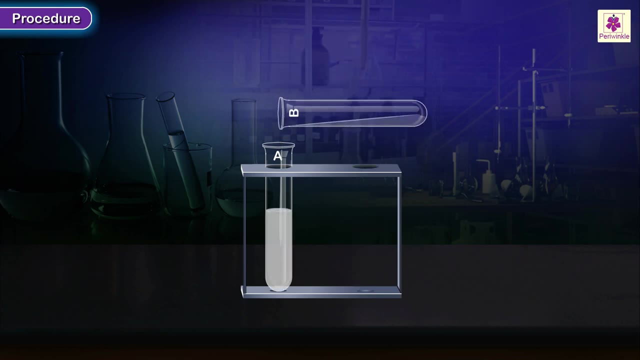 continuando Programme For the contents of one test tube into the other and observe the changes. if any, Instantly check whether there is any change or not. Please proceed with observation. When one solution is added to the other, instantly, you are able to check that an inference. 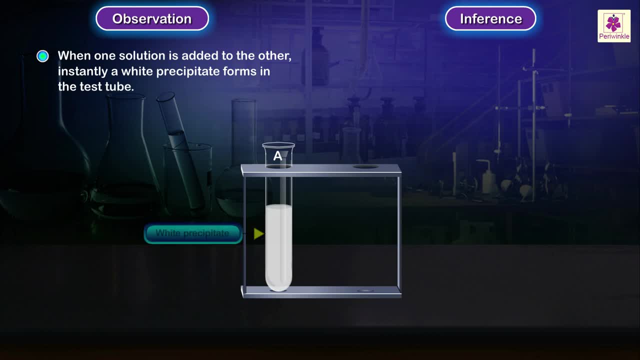 Add to the other a solution and compare the result without any error. DRENT C내. Drinh C altura, Salvador, Aundra. hoe white precipitate forms in the test tube, the reaction is instantaneous. in which at least one of the products is a white insoluble substance. procedure: leave the